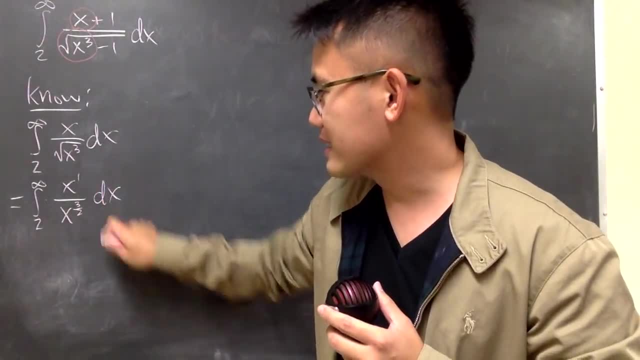 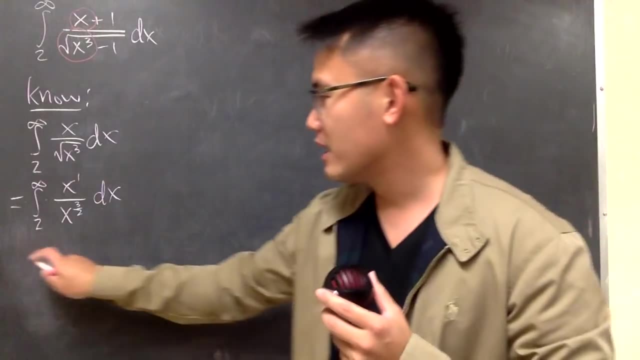 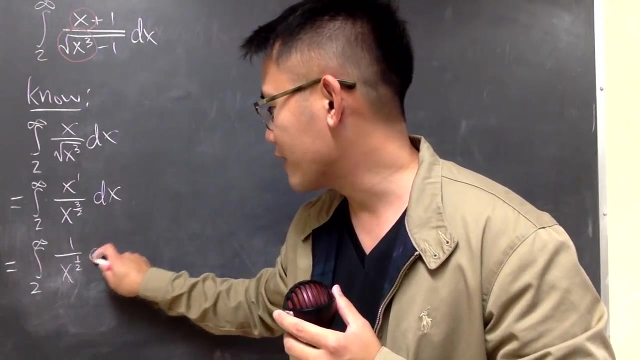 3 over the index 2, like this dx. And when we subtract the power 1 minus 3 half, We get negative 1 half. That means we can have this as the integral from 2 to infinity, 1 over x to the positive 1 half power, like that: 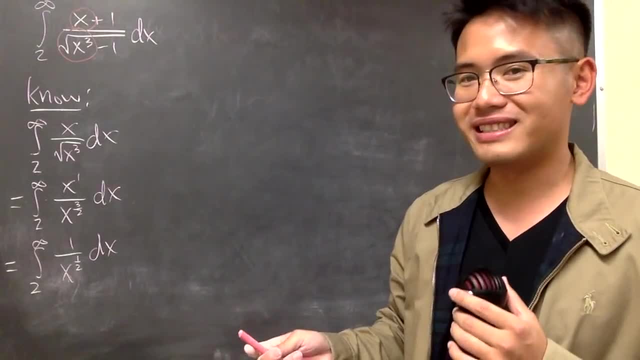 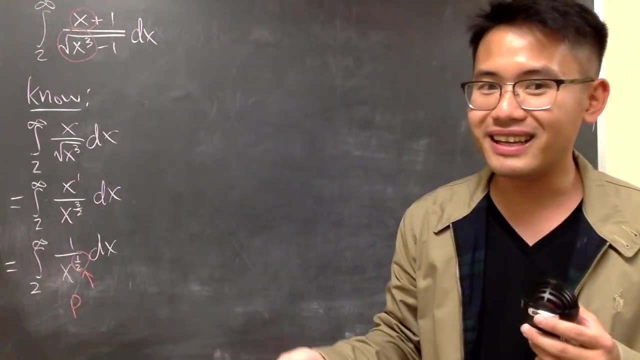 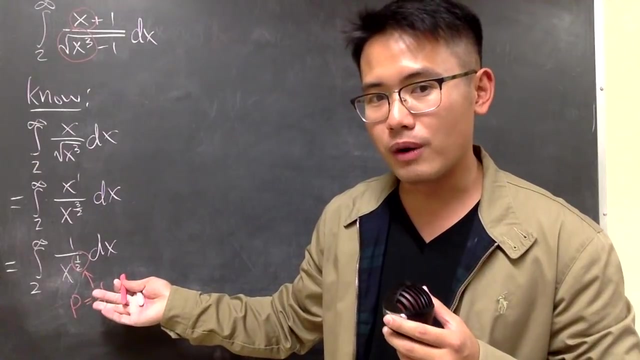 And when you have this you will actually know about this, Because you see that this right here is the p Right, this is the p integral for the p test. p right here is 1 half And this is the type 1 improper integral. 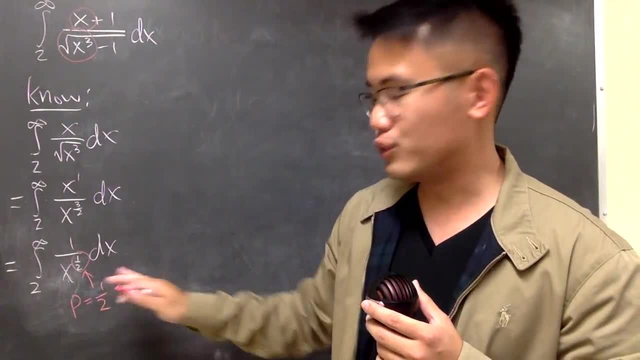 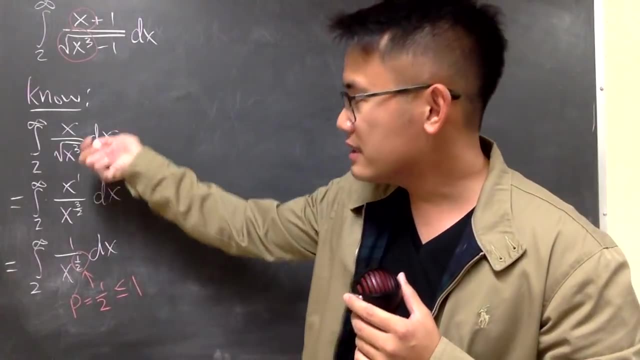 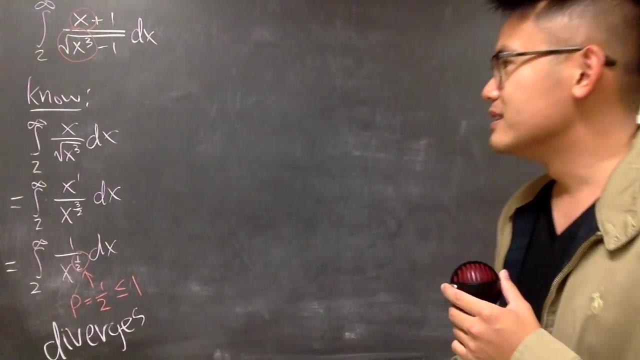 When p is less than or equal to 1.. Which we have, 1 half, It is less than or equal to 1.. This will tell us this improper integral actually diverges. Okay, So now, once you have this here, we are going to do the check. 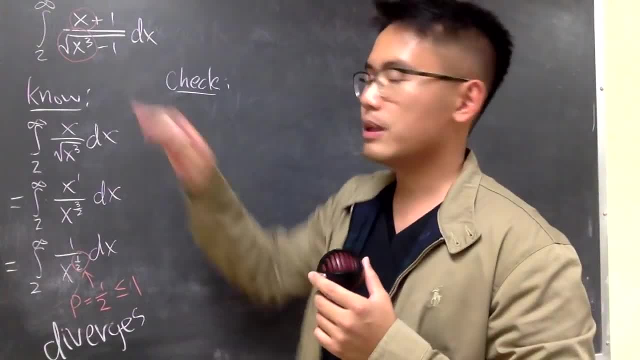 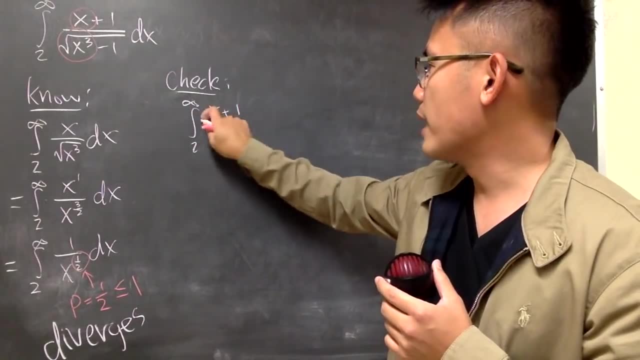 And, as what I've already told, you guys Put down the improper integral that you are trying to do on the left hand side, So let me write it down here: 2 to infinity x plus 1 over square root of x, cube minus 1, dx. 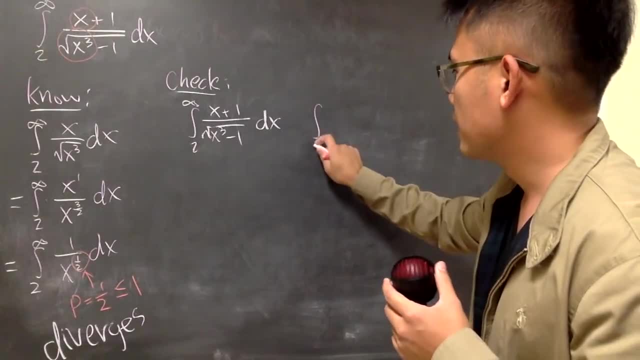 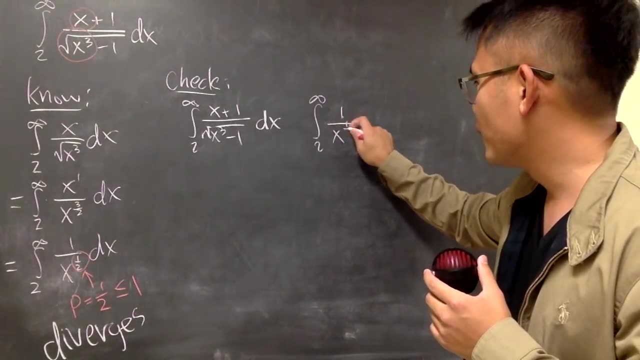 And put down the 1 that you know much better. on the right hand side And we are going to make a comparison And perhaps I will just put it down this form: 1 over x to the 1 half power dx, like this: 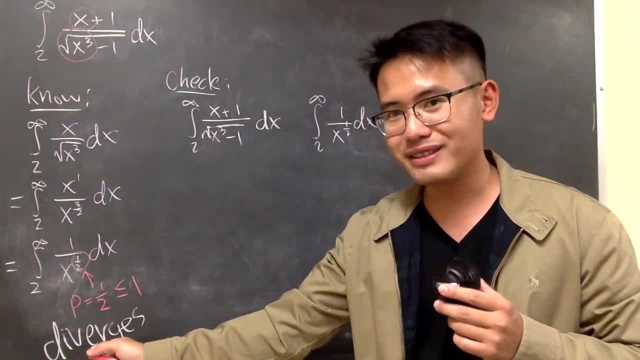 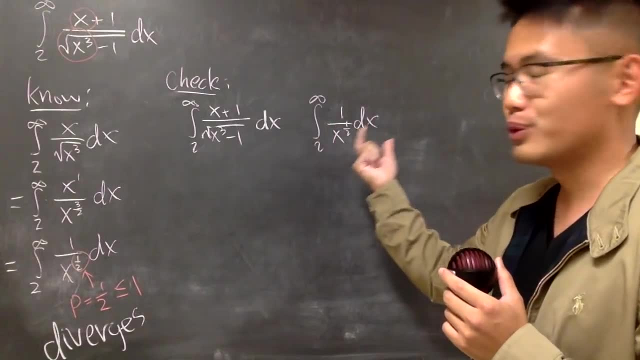 Remember this right here- diverges. It diverges to positive infinity. We actually want to show that if this is bigger than or equal to this right here, If we can show this is bigger than infinity, Of course this is infinity as well. 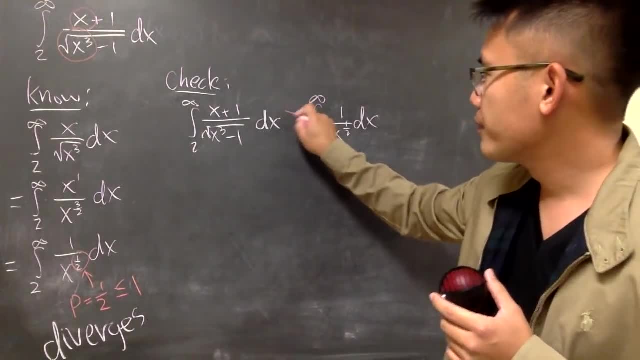 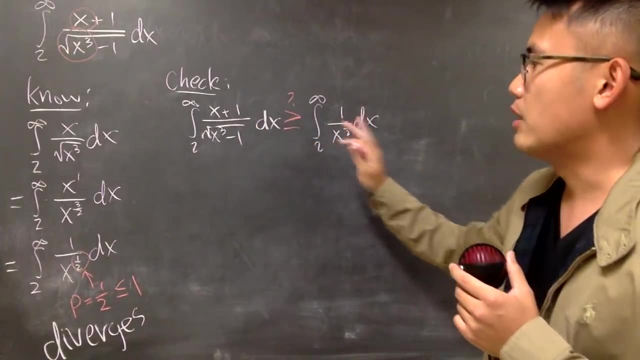 It's even a bigger infinity right. So we want to show this inequality. if it's true or not- And, by the way, both of this right here are positive- You guys can check that out, But you can indicate that on your own right here on the side. 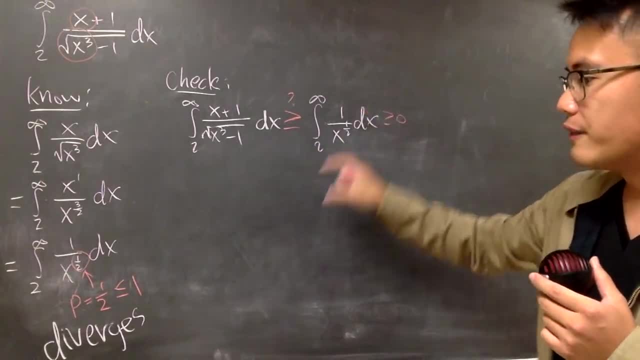 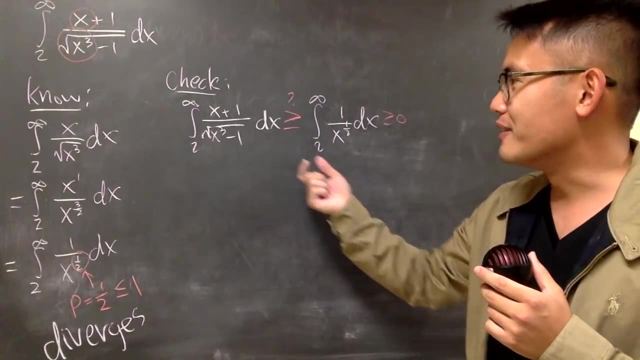 All the terms right here are positive And, once again, a diverge is like just like saying: if you meet somebody and you know this person is old, And if you can find somebody who is older than an old person, what can you say about this person? 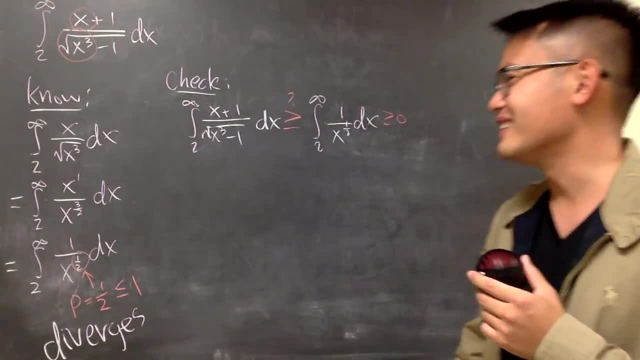 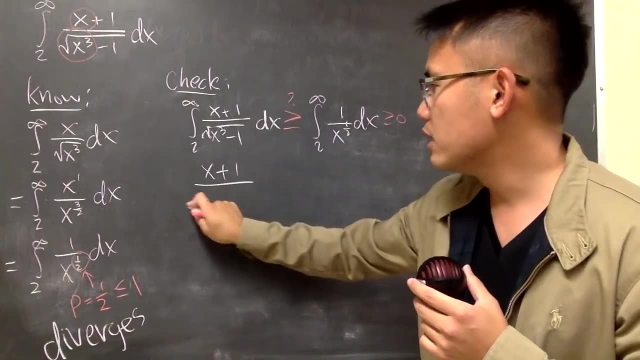 He is also old, right, So that's pretty much the idea. Anyway, let's do the algebraic check, Because now we just have to worry about the function part. This is x plus 1 over square root of x, cube minus 1.. 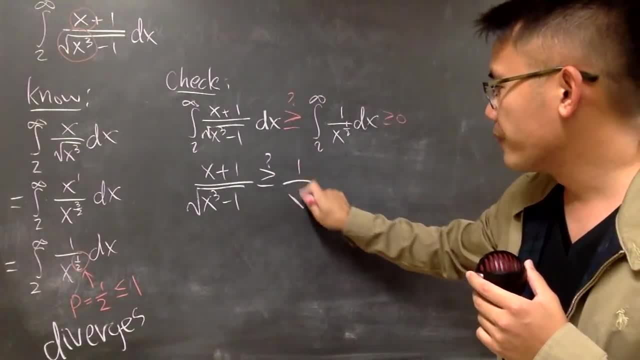 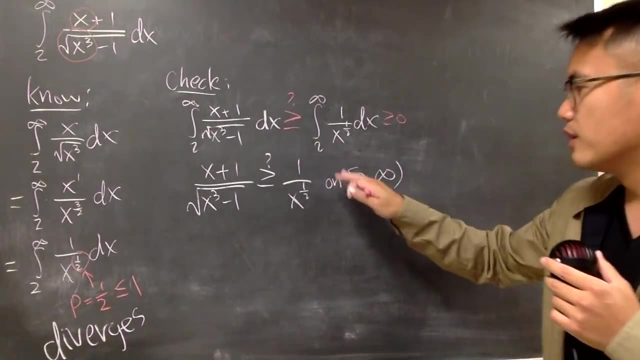 I want to see if this is bigger than or equal to 1 over x to the 1 half on the interval 2 to infinity. Or you can also write: 4x is greater than or equal to 2.. Doesn't matter, same thing. 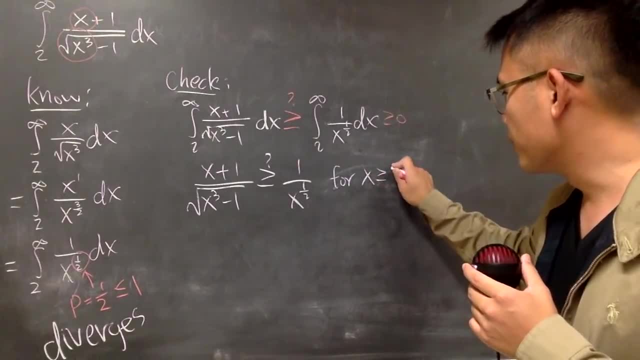 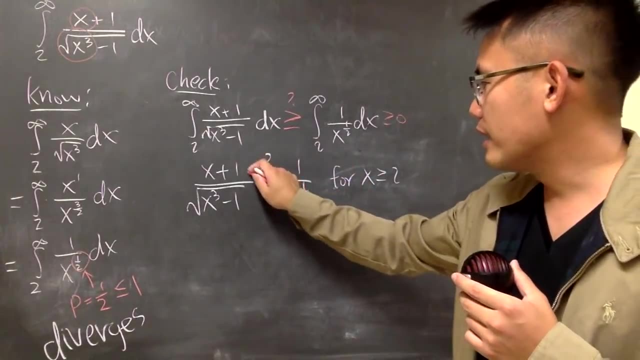 Perhaps I will do that. 4x is greater than or equal to 2. Because we go from 2 to infinity. Okay, everything is positive as indicated here, So I can cross multiply Without changing the inequality symbol, And let me just do this times that. 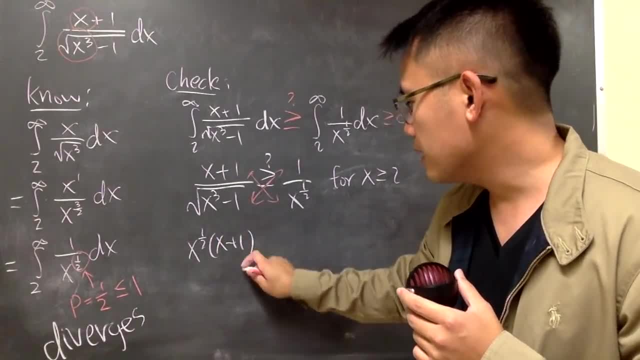 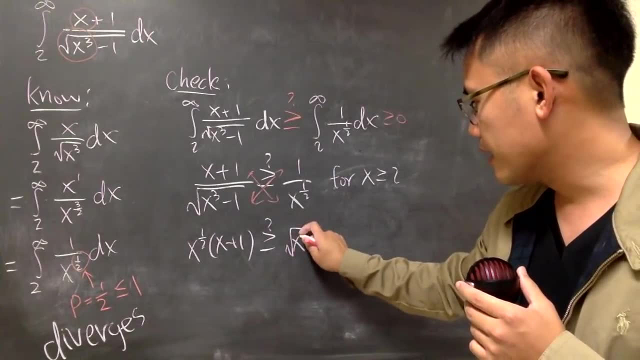 Which is x to the 1 half times x plus 1.. Multiply this- and that I don't know yet, so I will put on the equation mark- And then we have the x cube minus 1.. Well, I have the square root. 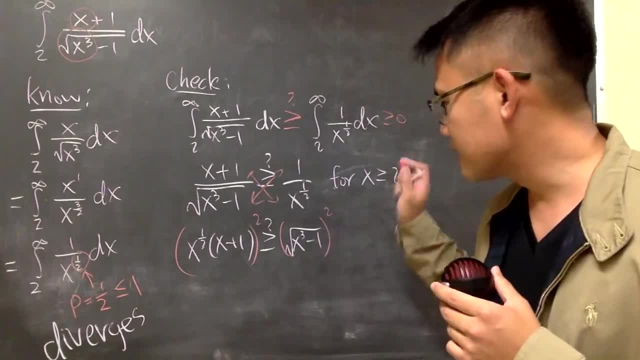 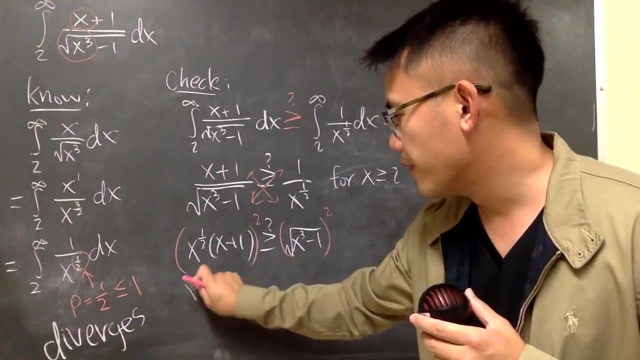 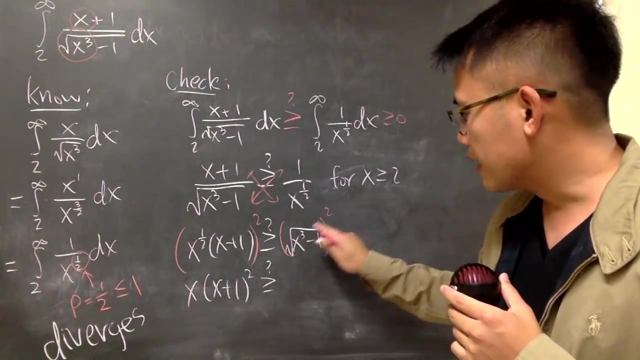 I don't like that. Perhaps I will square both sides And you see, distribute the power. in this case, you get x to the first And then you have x plus 1 square. Is this greater than or equal to? Cancel this out. 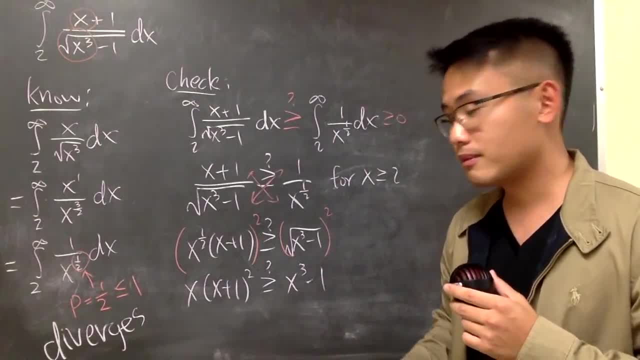 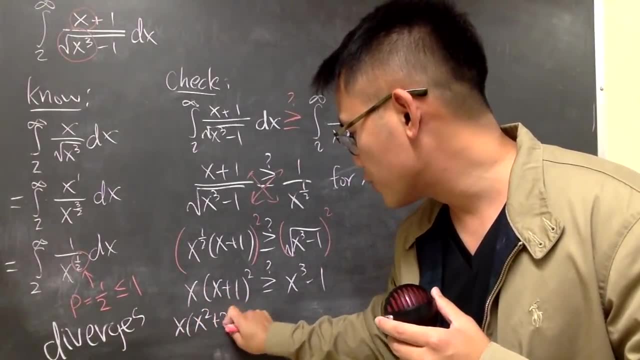 x cube minus 1.. Well, if you would like, you can do more algebra right here. right, Expand this, you have x in front. Expand it, you get x square plus 2x plus 1.. Is this greater than or equal to x cube minus 1?? 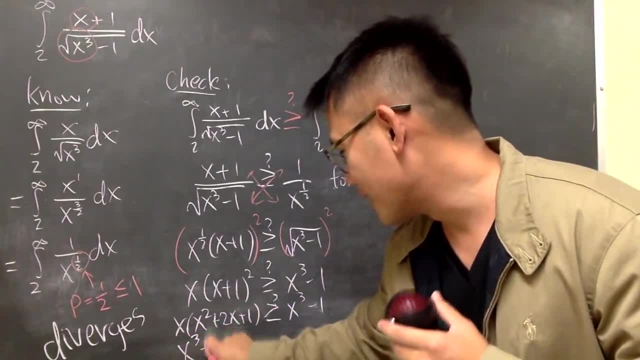 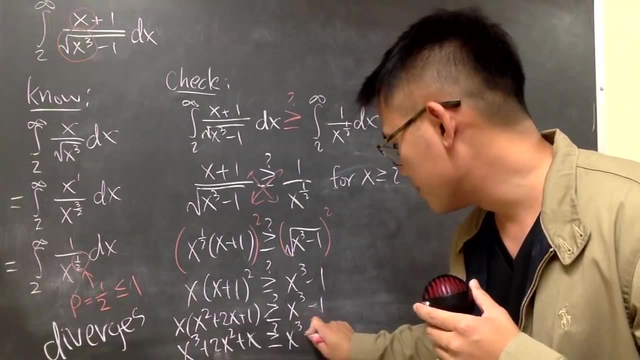 If you would like, you can distribute x cube plus 2x plus 1.. 2x square right And then plus x. Is this greater than or equal to x cube minus 1? This is my question mark, by the way. 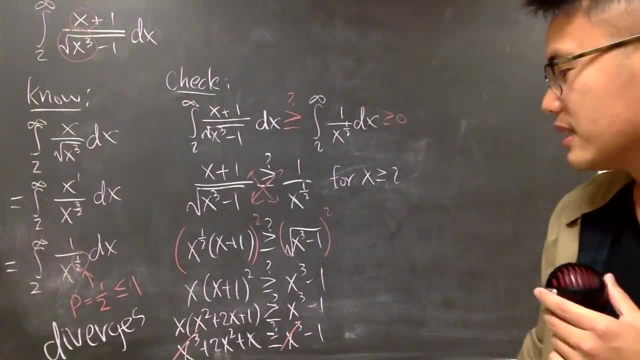 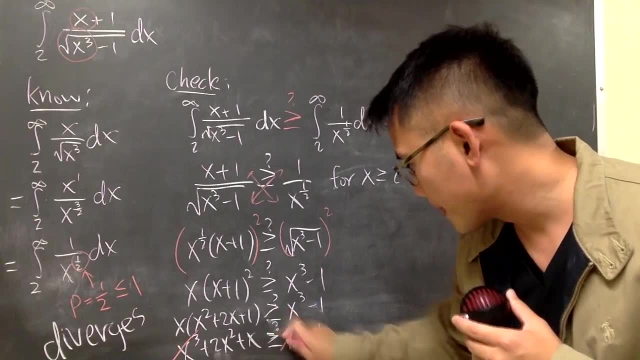 I think so, Because you can totally cancel out the x cube on both sides And you have 2x square plus x. It is greater than or equal to. It is greater than or equal to negative. 1. Because you have x is greater than or equal to 2..